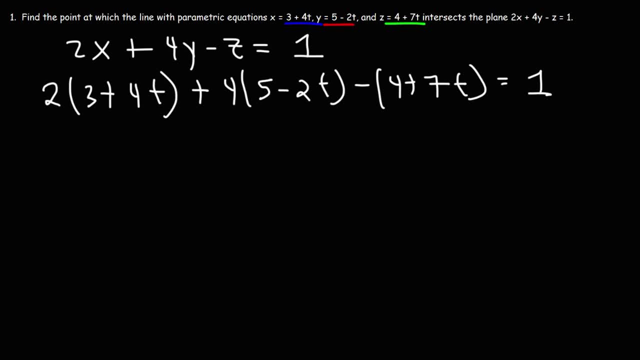 Now the next thing we need to do is solve for t, But let's distribute first. So we have 2 times 3, which is 6. And then 2 times 4t, that's 8t. 4 times 5 is 20.. 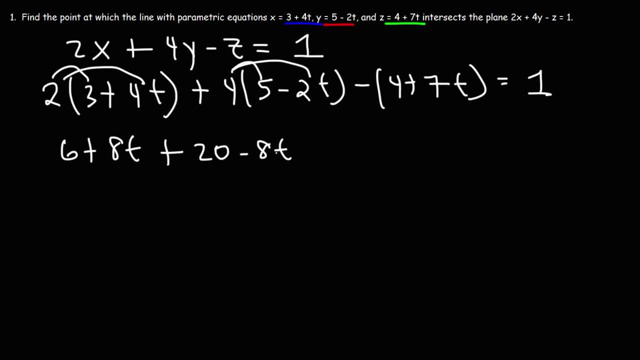 4 times negative 2t, that's negative 8t, And then we need to distribute the negative side, So this is going to be minus 4, and then minus 7t, Which is equal to 1.. Now let's combine like terms. 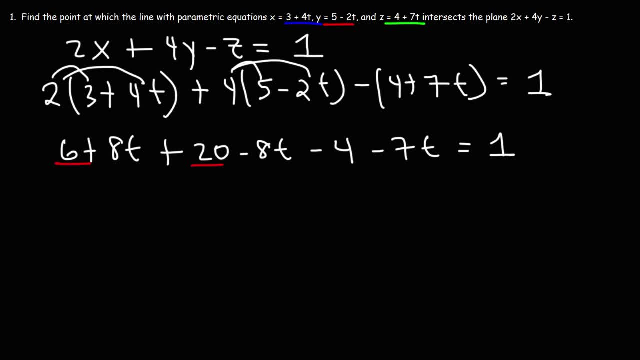 So we have 6 plus 20,, which makes 26, minus 4.. So that's 22.. 8t and negative 8t will cancel, So we're left with this. Our next step is to subtract both sides by 22.. 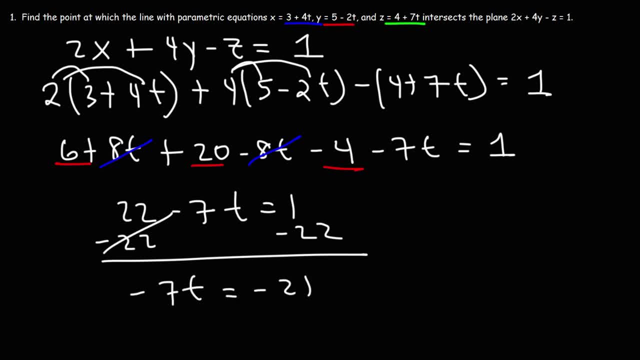 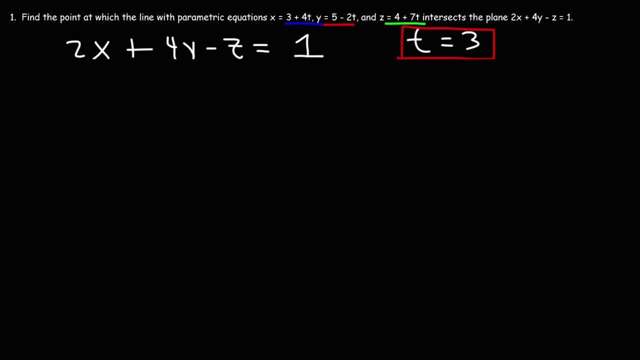 1 minus 22 is negative 21.. And then we need to divide both sides by negative 7.. So negative 21 divided by negative 7 is 3.. So t is equal to 3.. Now the next thing that we need to do is take our t value and plug it in to the parametric equations. 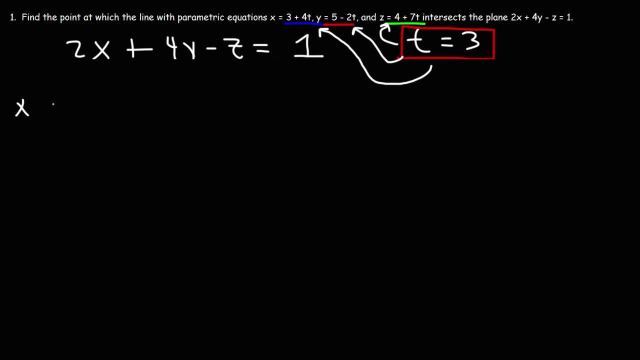 This is going to give us x, y and z, So let's start with the first one. x is equal to 3 plus 4t, So that's going to be 3 plus 4 times 3.. 4 times 3 is equal to 3.. 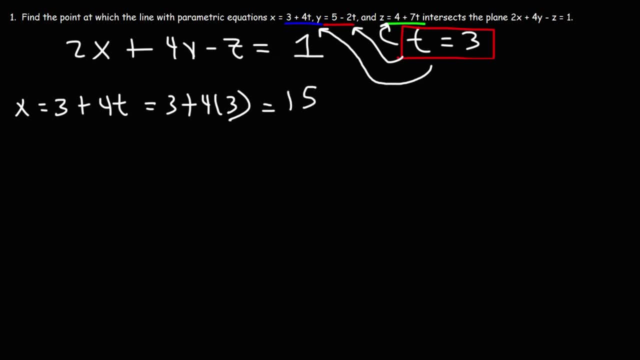 4 times 3 is equal to 3.. 4 times 3 is 12 plus 3.. That's 15.. So next we need to calculate y. So we have 5 minus 2t, And this is going to be: 2 times 3 is 6.. 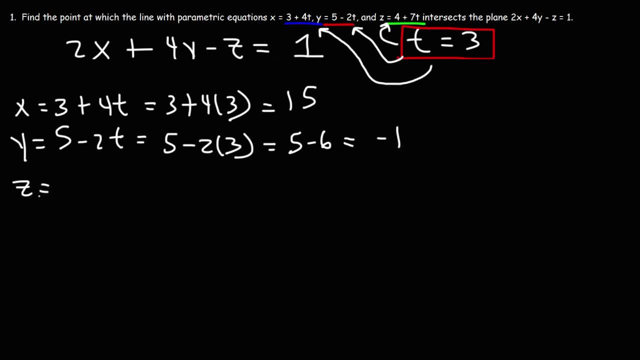 5 minus 6 is negative 1.. Next we have z, which is 4 plus 7t, So that's going to be 4 plus 7 times 3.. 7 times 3 is 12.. And then 4 plus 7 is 21.. 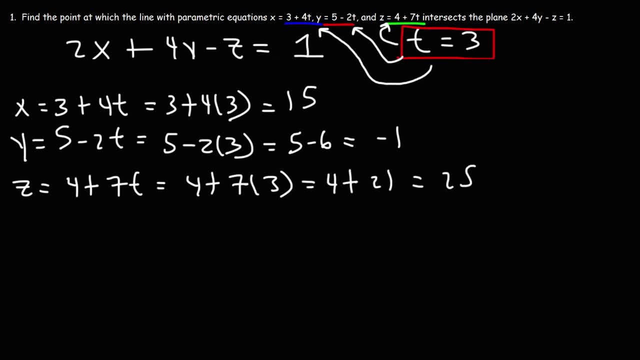 And then 4 plus 21 is 25.. So we have x, y and z. So the answer is going to be 15 comma negative, 1 comma 25.. So this is the point of intersection between the line and the plane. 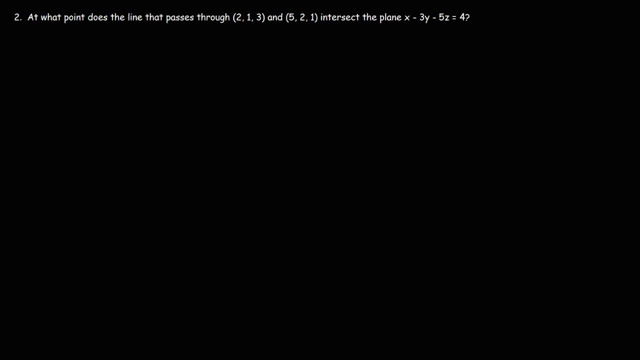 So that's how you could find it. Now let's move on to the second type of problem that we can encounter. So, with this type of topic, At what point does the line that passes through 2 comma 1, comma 3 and 5 comma 2 comma 1 intersect? the plane x minus 3y minus 5z equal 4?. 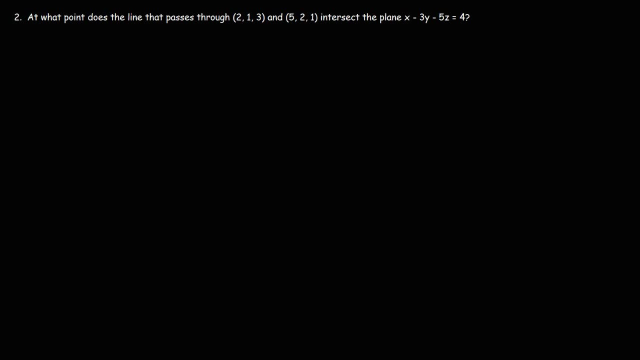 So this problem is a little different. But if we can find the parametric equations of the line that intersects the plane, then we can do what we're going to do. We're going to do what we did in problem 1.. So that's what we need to do in problem 2.. 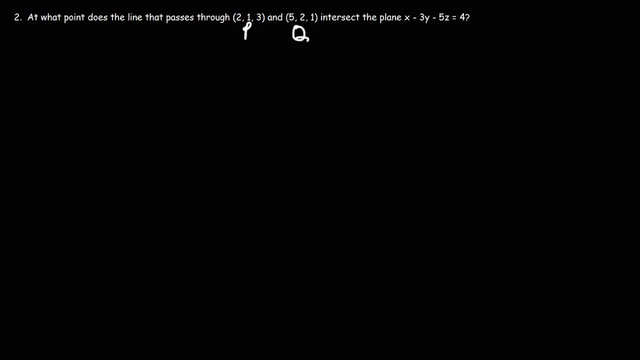 Let's call this point p and point q. In order to define a line, we need a point and a vector. So let's find a vector, which we'll call vector pq. So we're going to subtract point q from point p. 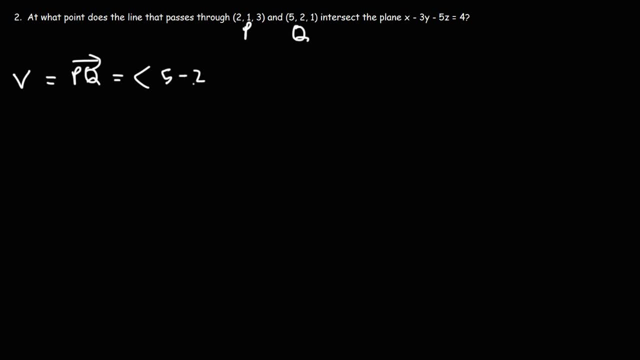 So it's going to be q minus p. So we're going to subtract q. So we're going to have 5 minus 2 comma, 2 minus 1 comma, 1 minus 3.. So we're subtracting the x values, the y values and the z values. 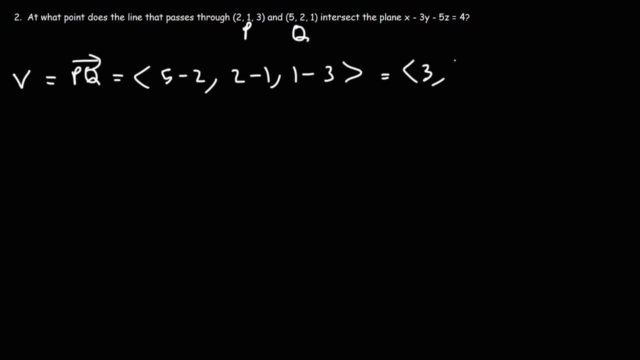 So 5 minus 2 is 3.. 2 minus 1 is 1.. 1 minus 3 is minus 2.. So that is the direction of the line which is defined by vector v. Now what do we do? 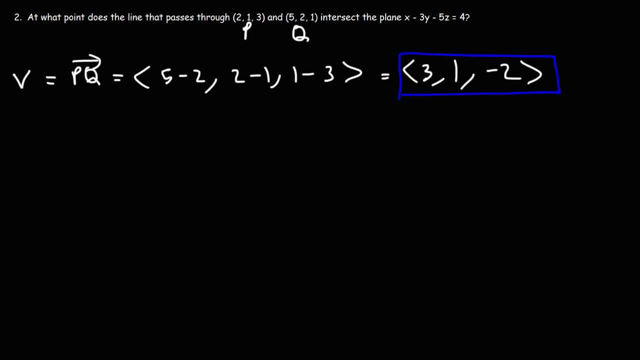 At this point, we're going to subtract the x values. At this point, now that we have the vector, how can we write the parametric equations for this line? Here are the formulas that you need: x is equal to x sub 0 plus a t. 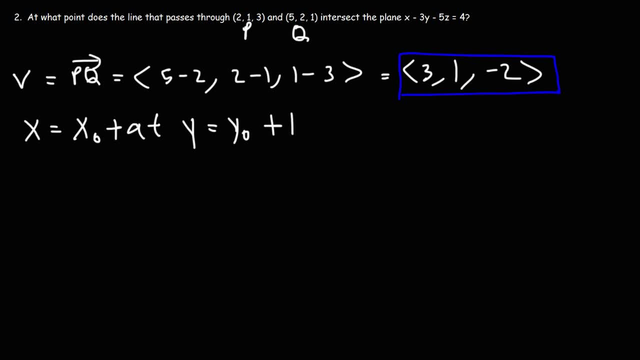 y is equal to y sub 0 plus b t, And z is equal to z sub 0 plus c t. So vector v tells us or gives us the values that we need, And vector v tells us, or gives us the values that we need. 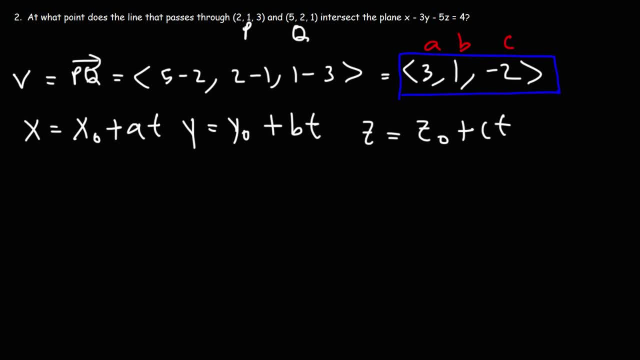 a, b and c. Now to find x, y and z sub 0, we need to choose one of the two points that we have, either point p or point q. So let's use point p. x 0 is going to be 2, y 0 is 1, z sub 0 is 3.. 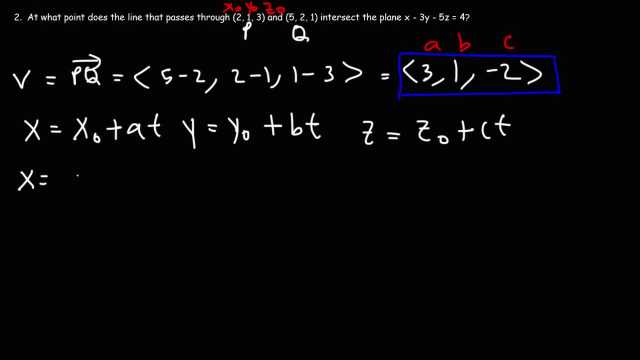 So we're going to have: x is equal to x sub 0 is 2, a is 3.. So x is equal to 2 plus 3t. y sub 0 is 1, b is 1.. So that's just going to be 1t or just t. z sub 0 is 3, c is negative 2.. So 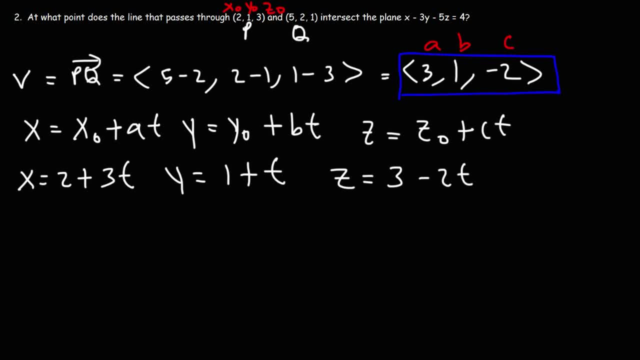 this is going to be 3 minus 2t. So here are the parametric equations that define the equation, The line that passes through the points 2, 1, 3, and 5, 2, 1.. So now let's start with the equation of the plane. So x minus 3y minus 5z is equal to 4.. 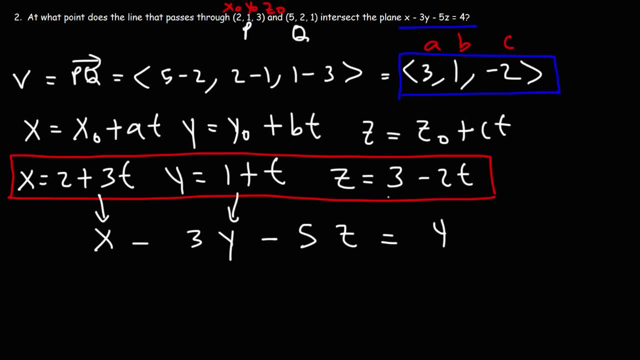 Now let's plug in x, y and z into that equation so we can get an equation that contains only the t variable. So this is going to be 2 plus 3t minus 3 times 1 plus t minus 5 times 3 minus 2t. So now let's do some algebra. 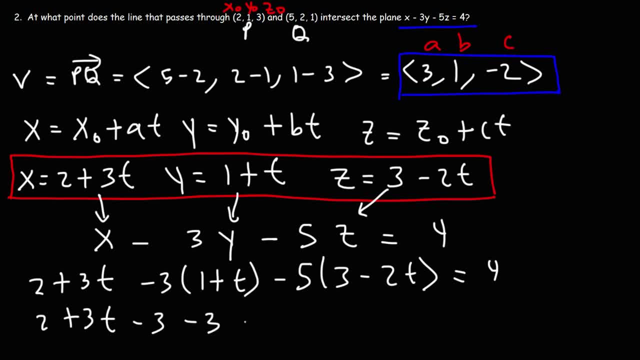 Let's distribute the negative 3.. So this is going to be minus 3 minus 3t, and then distributing negative 5.. Negative 5 times 3 is 15.. Negative 5 times negative: 2t, that's positive 10t.